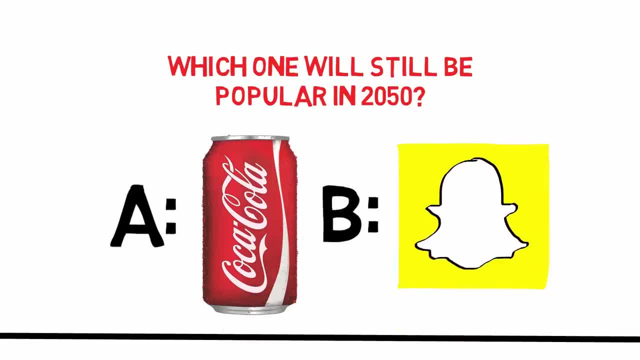 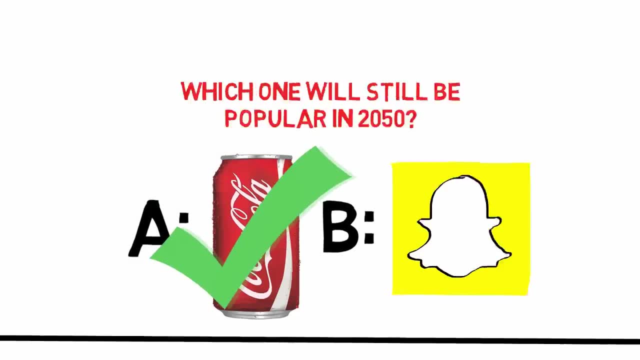 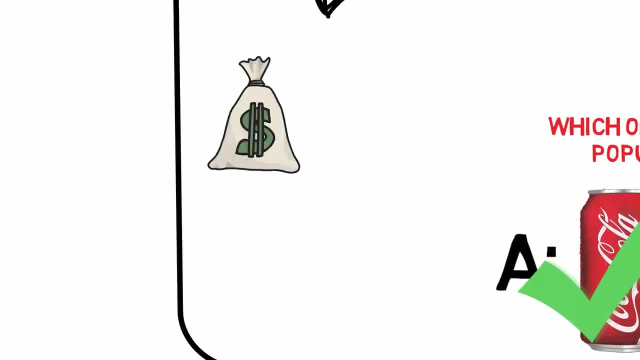 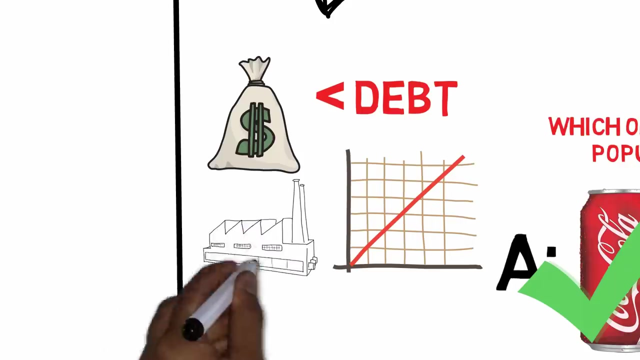 Snapchat, Which has been popular for about seven years. The answer is quite obvious. When Warren Buffett is looking for investments with a sustainable competitive advantage, he wants to see consistency: Consistency in earnings, consistent low debt, consistently growing earnings, consistently low spending in capital expenditures and R&D. 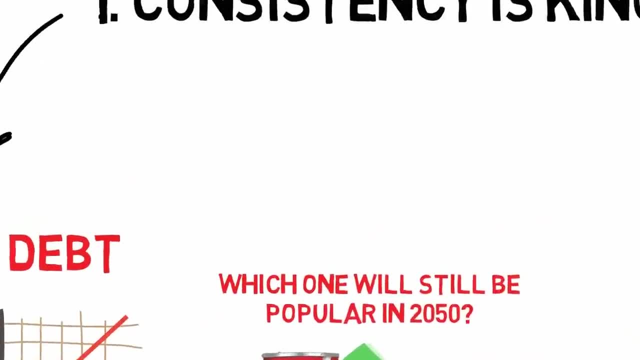 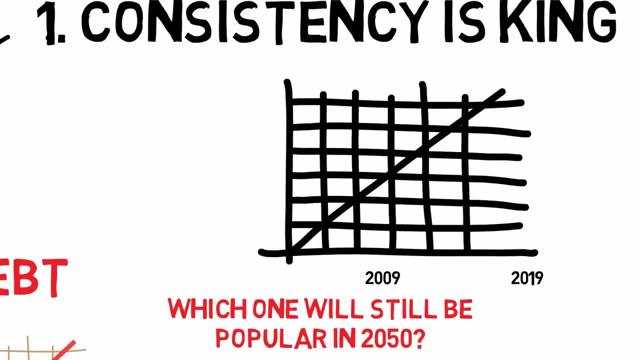 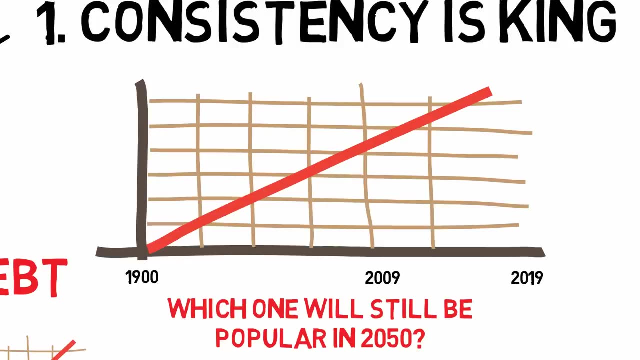 consistent profitability, etc. To look at the last 10-year period is a good start But, as in the case of Coca-Cola, the longer the company has been proving its durability, the better. Selling the same product for many years, such as Coca-Cola has done, has a great advantage for you as the stock owner. 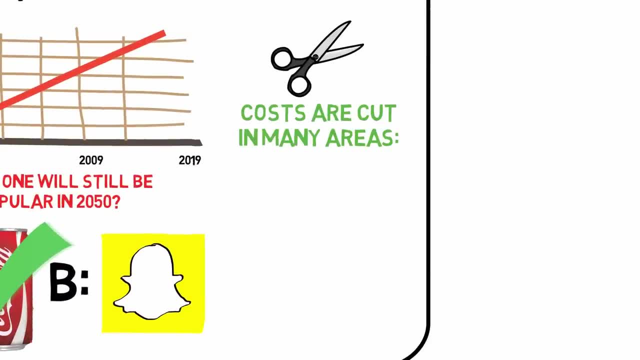 It reduces costs by a lot. It reduces production costs, as the need to upgrade machinery decreases. It reduces marketing costs, as marketing efforts are cumulative. It reduces costs for research and development Duh It lowers the training cost of employees. It reduces the risk of having obsolete inventory. 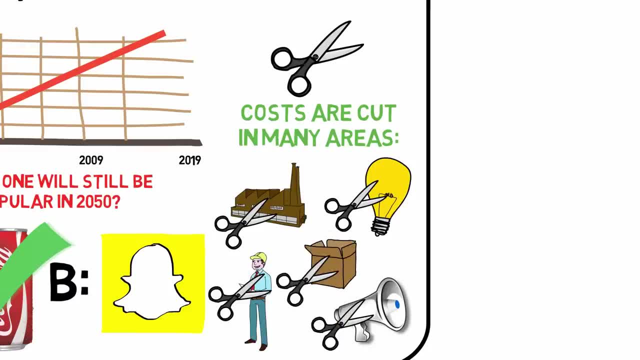 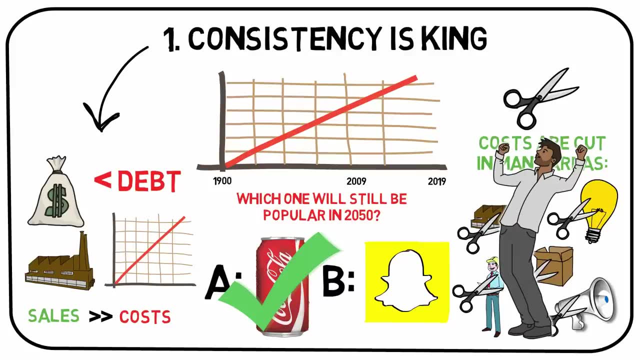 And when costs are reduced by a lot, it means a lot more money in the pockets of shareholders. Not only are the costs reduced in these companies, But you'll be able to experience compound interest tax-free when your holding period is forever, Which is something that has made Warren Buffett awfully rich during the last 50 years. 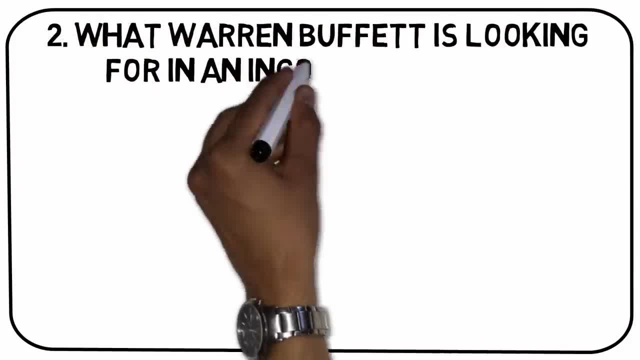 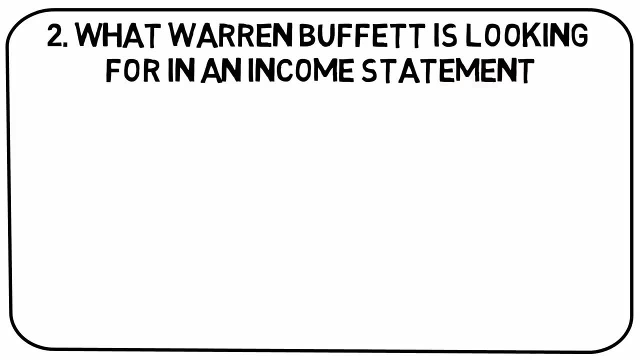 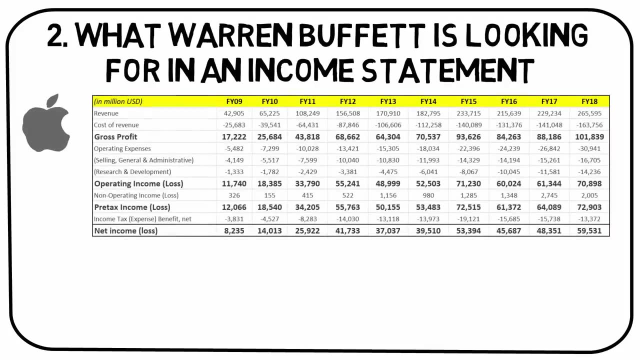 Takeaway number 2: What Warren Buffett is looking for in an income statement. To illustrate what Buffett looks for, we will use one of his more recent and largest investments: Apple. First and foremost, I will assume that you know some basics about Financial statements If you don't head over to my summary of the interpretation of financial statements by Benjamin Graham for some investing 101. 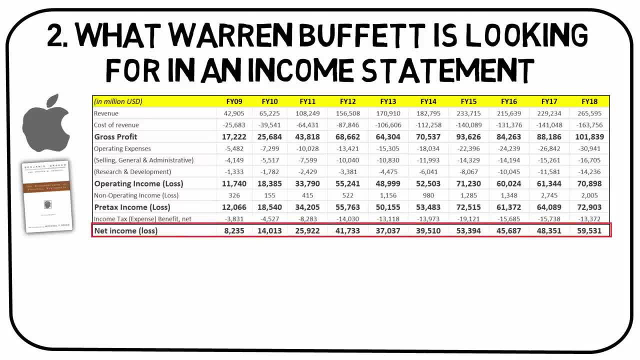 Let's start out by having a look at the bottom line to confirm what we talked about in the previous takeaway. The net earnings of the company has shown great consistency over the last 10 years. Fair enough. it doesn't have the track record of Coca-Cola, and neither are its products as durable in my opinion. 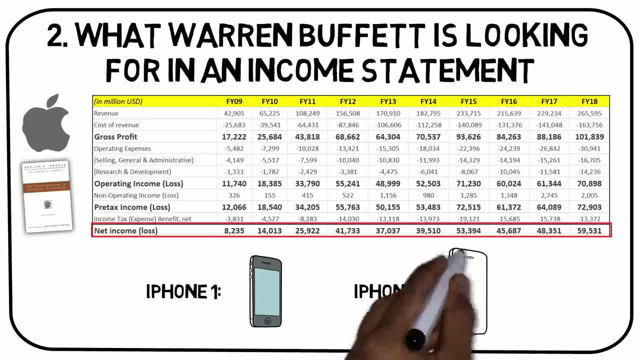 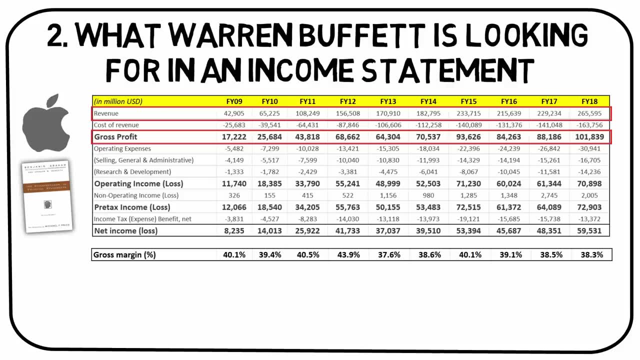 But the iPhone has looked quite similar since its release in 2007. Moreover, the earnings of Apple have grown at a steady pace. Another thing that Warren Buffett wants to see in his investments is a consistent and high gross margin. As a rule of thumb, you'd want to see a margin of 40% plus. 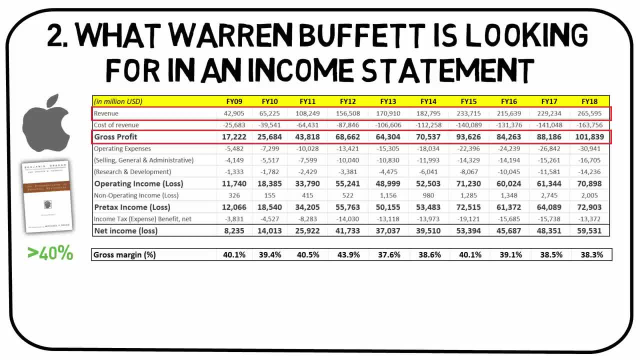 We can see that Apple just makes the cut here. It's always interesting to compare with competitors as well. So, as a point of reference, Samsung had a gross margin of 45.3%- 7% in 2018- and Huawei had a margin of a 38.6%. 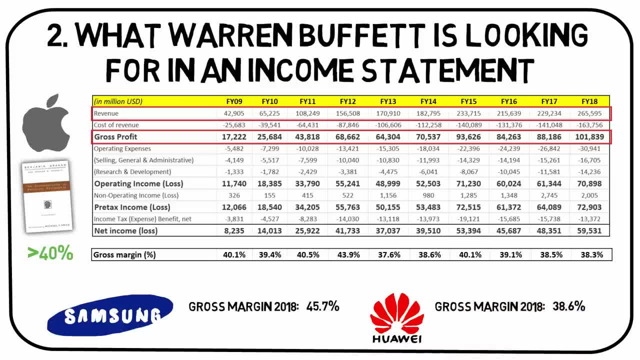 Having a high gross margin typically says something about the scalability of the business, Meaning that the more the company sells, the greater the profitability becomes. This is the trait that you'd want to see in any business that you own. Finally, we want to compare the bottom line to the top line and calculate the net margin. 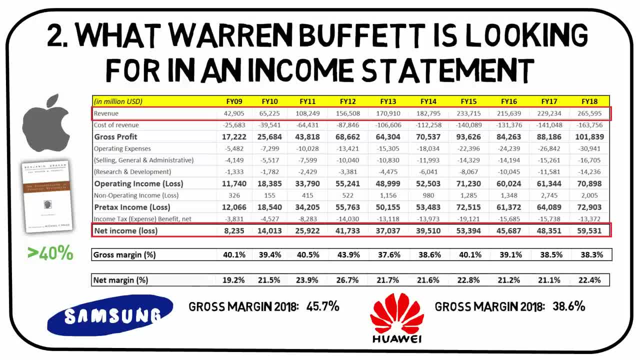 Companies with a durable competitive advantage have higher net margins than their competitors. Apple beats both Samsung and Huawei in this regard, And here's another rule of thumb: A net margin of 20% or higher is typically a very strong result, Revealing that we are dealing with a smoothly run business. 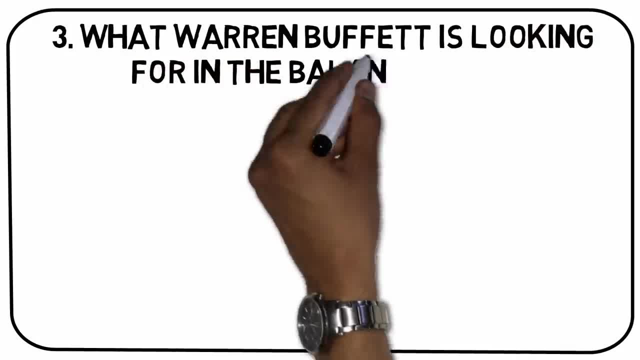 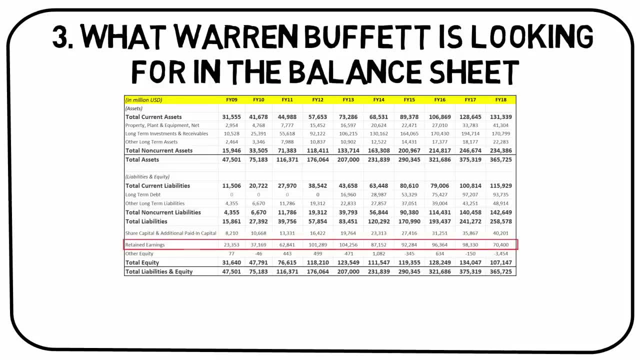 Takeaway number 3: What Warren Buffett is looking for in the balance sheet. Next up is the balance sheet Warren Buffett likes to look at a figure called retained earnings. The figure is being added to or withdrawn from each year, depending on if the company is reinvesting its net income or not. 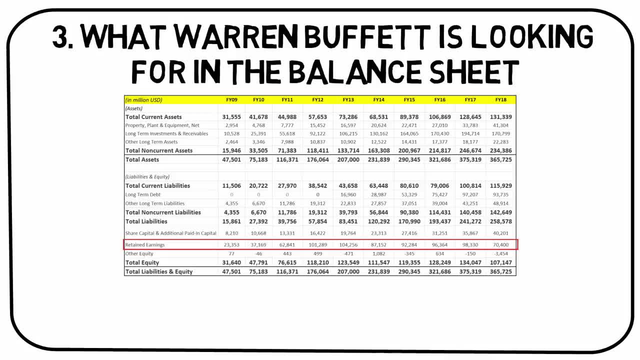 Buffett typically likes to see a steady growth here, Meaning that the business is profitable and that it identifies good reinvesting opportunities. If we look at Berkshire Hathaway's retained earnings, for example, we see a very strong growth during the last decade. Apple doesn't really fulfill the criterion regarding retained earnings. 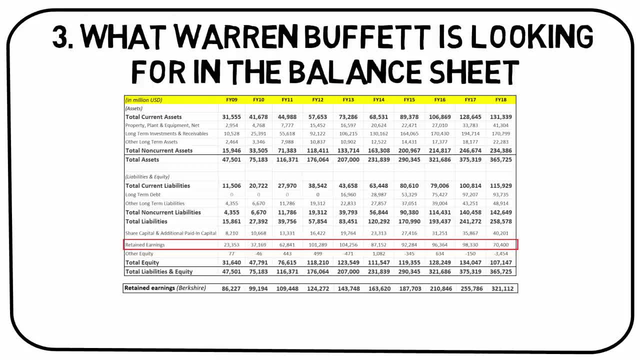 But one must also take into consideration that, Starting in 2013,, Apple began a quite extensive dividends and share repurchase program. We'll get to this in the next takeaway. To measure how efficient a company is using these reinvested earnings, return on equity can typically be used. 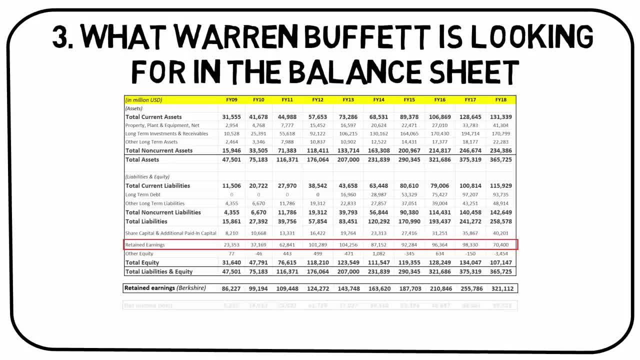 To calculate this, we must revisit the income statement and compare the net income to the total equity of the company. Apple is showing a lot of strength in this regard, Which is partly an effect of distributing so much of the earnings to shareholders, But also a sign of a business with a durable competitive advantage. 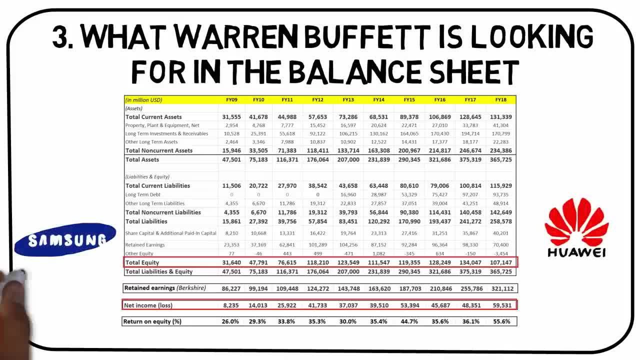 As a comparison, Samsung and Huawei aren't even half as profitable. In his 1983 shareholder letter, Warren Buffett suggests a somewhat more sophisticated approach towards measuring How efficient a company is using its capital. He suggests that one should calculate the so-called return on net tangible assets. 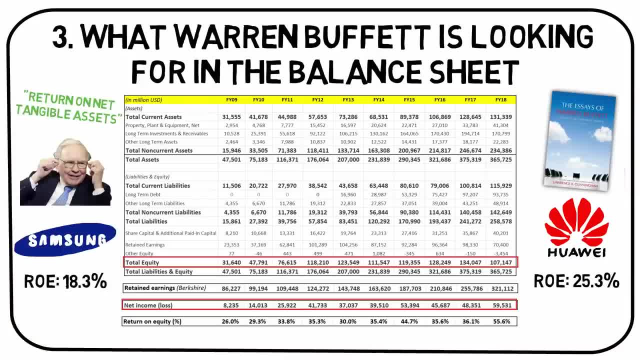 More on this in the essays of Warren Buffett. A third thing to notice is that the exceptional business seldom requires a lot of debt to expand, Banks perhaps being the exception, Because usually it can just use the strong cash flow from the business. Therefore, look for businesses with little to no long-term debt. 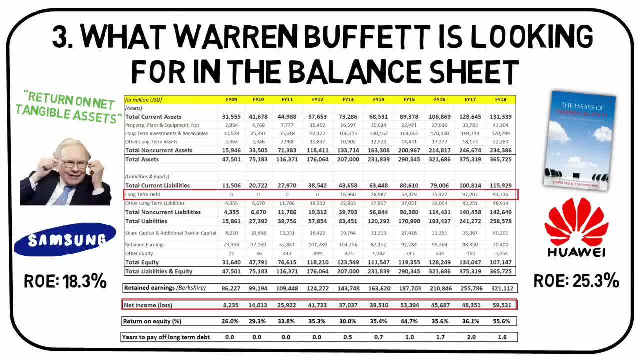 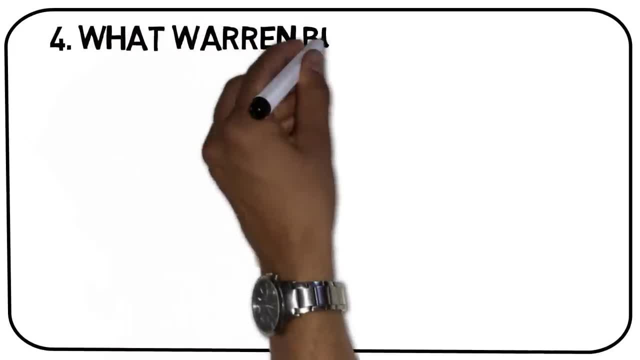 If a company can pay off all its long-term debt with less than four years of earnings, it's in quite a good position. Apple clearly fulfills this criterion, and its competitors do too. Takeaway number 4. What Warren Buffett is looking for in a cash flow statement. 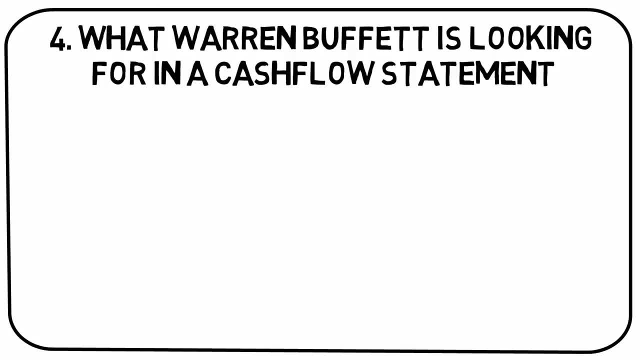 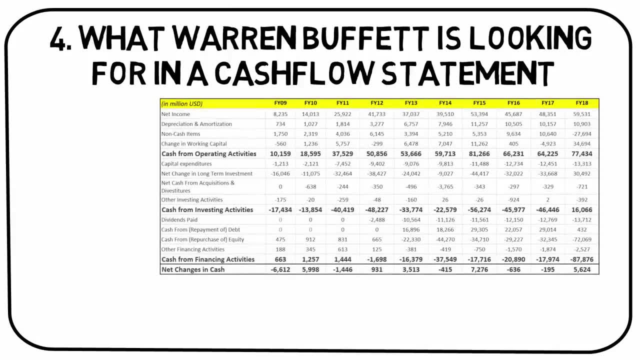 Finally, the third financial statement that you must dive into is the cash flow statement. A cash flow statement differs from an income statement in that it represents actual ins and outs of money, While the income statement is a measure of financial performance. Yes, I will probably make a video of its own about this in the future Comment. 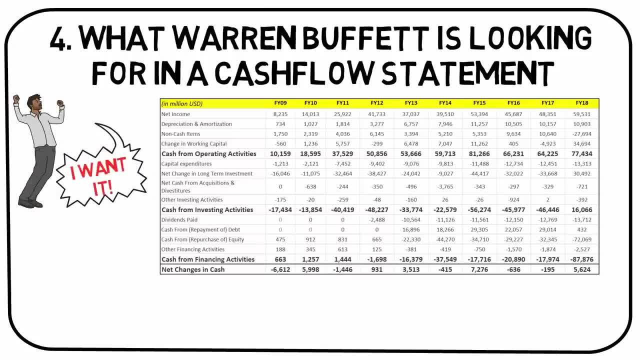 I want it down below, if you. well, if you want such a video, For now, It's enough that you know that one important figure is the capital expenditures. This is money being spent on properties, plant and equipment. primarily, Look at what percentage capital expenditures are of net earnings. You want them to be as low as possible. 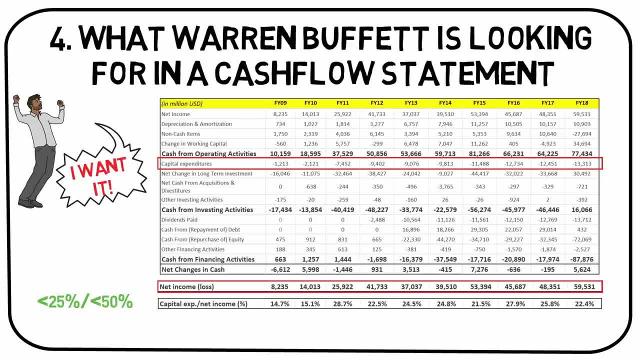 Lower than 25% over a period of time is considered very good, and less than 50% is acceptable. There are exceptions, though, such as when a company is making a one-time payment to grow the business. Look at what the company is using the money for. 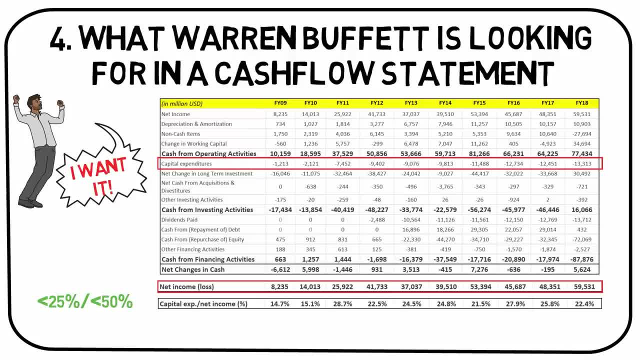 Apple does very well here. In almost every year They had capital expenses at less than 25%. The same thing can't be said about its competitors. Also, in the cash flow statement, We can see the reasons why the retained earnings from the balance sheet haven't been growing much since 2012. 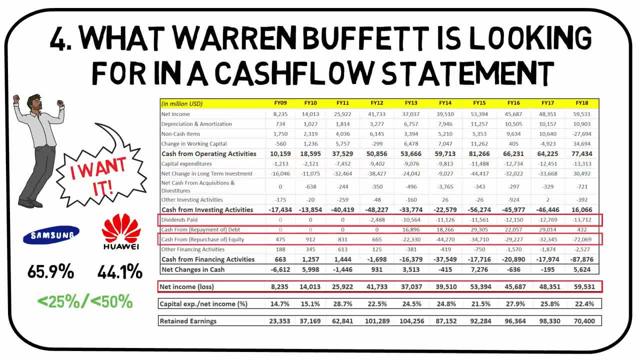 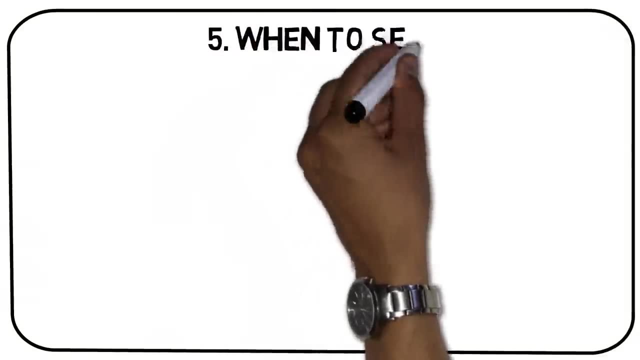 Apple has been distributing a lot of cash to its shareholders. The so-called augmented payout ratio, which includes share buybacks as well as dividends, has been higher than a hundred percent during some years, Which basically means that Apple is distributing more money than it earns. Takeaway number 5. When to sell. 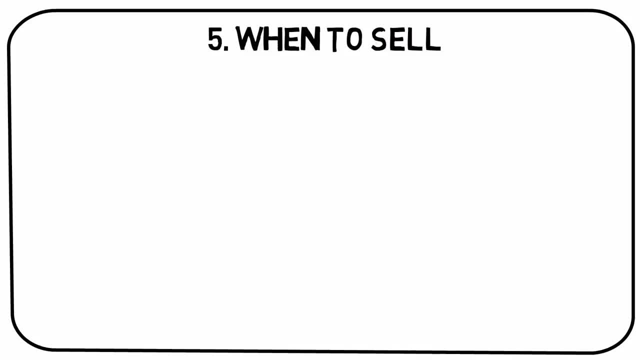 As I've talked about before, one of Warren Buffett's key concepts on how to invest in stocks successfully is to hold on to your investments forever. Still, though, there are three instances when you might consider selling your stock. 1. You need more money for your investments. 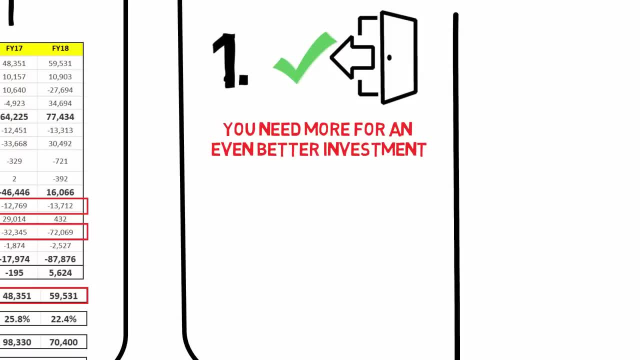 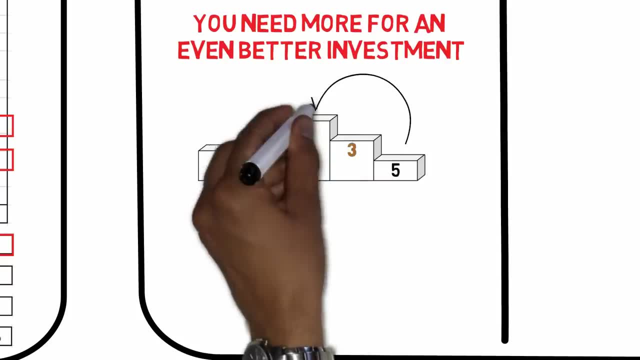 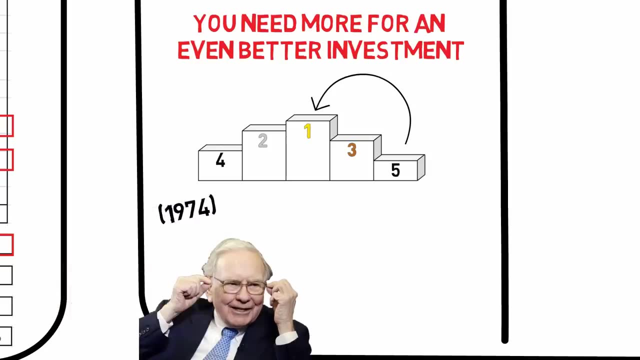 2. You need more money for an even better investment. At times, perhaps, especially in bear markets, there are so many opportunities to go around that you must consider switching from something that is great to something that is exceptional. In 1974, Warren Buffett said this, noting that a lot of stocks were undervalued. 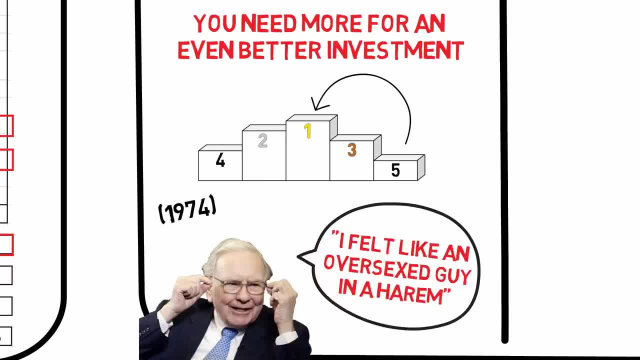 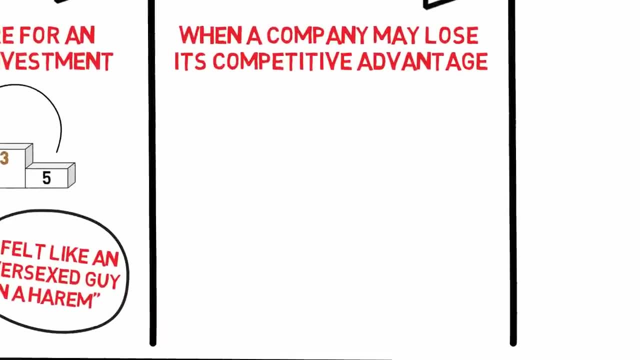 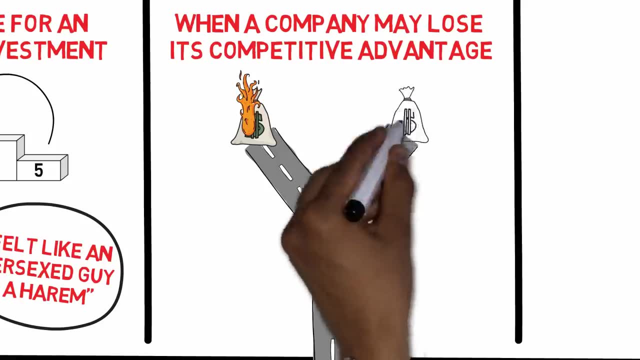 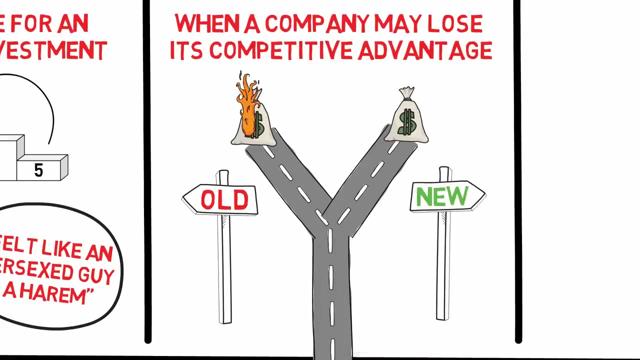 I felt like an over-sexed guy in a harem. 2. When a company may lose its competitive advantage. Times are changing. For example, the once monopoly-like characteristics of the local newspapers are now being disrupted by online media. If one of your investments face a risk of this kind, it may be time to cut it loose. 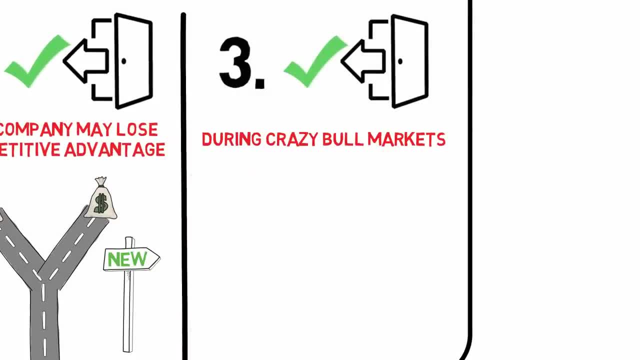 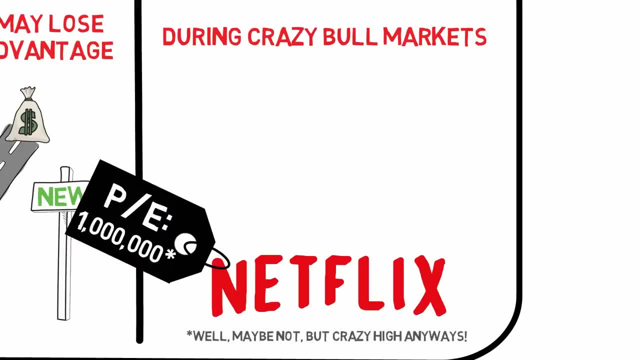 3. During crazy bull markets, Even a fantastic business can be a bad investment if you must acquire it at a crazy price, And likewise, there are times when you can improve your personal finances by selling a fantastic business at such a price if you are already holding on to one. 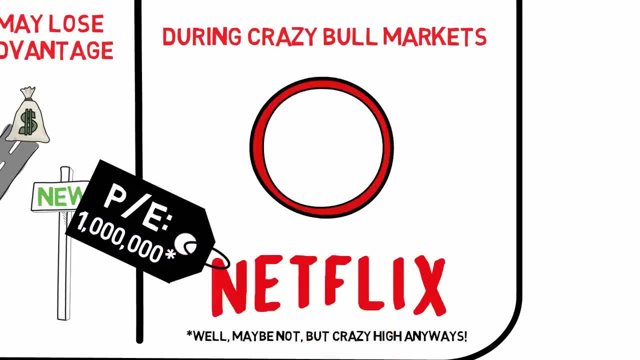 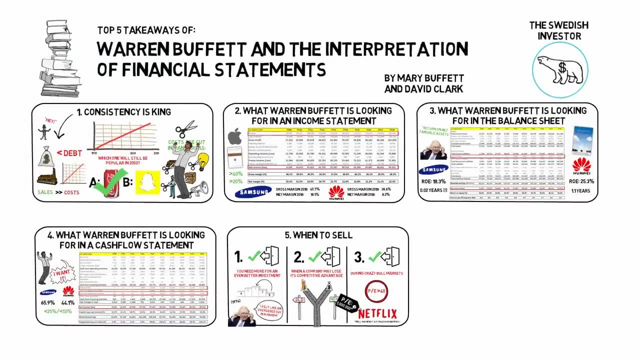 Mary Buffett and David Clark suggest that, at a P-E ratio of 40 or higher, you should start consider selling your stocks, even if you believe in the underlying economics of the company. And that's it, A quick summary. When you are looking for a business with a durable competitive advantage, the key word is: 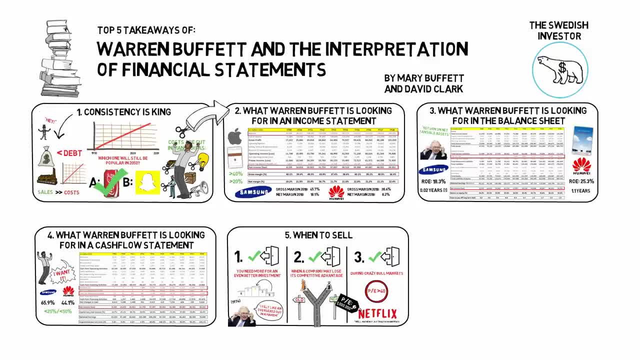 CONSISTENCY In the income statement. look for consistently growing net earnings and profit margins that consistently beat the competitors. When observing the balance sheet, remember that the superior business has a higher return on capital, that it seldom requires a lot of debt and.